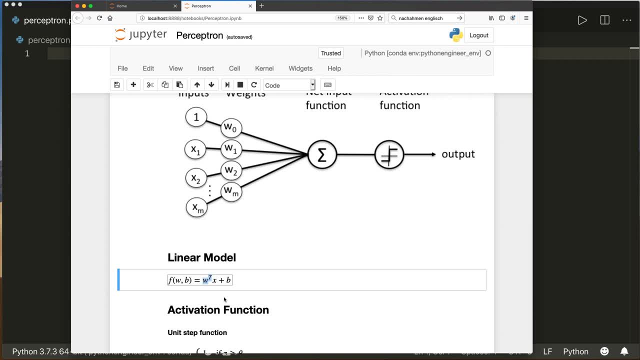 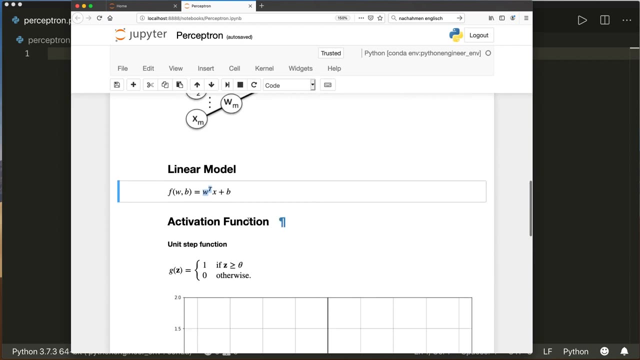 up our weights and the bias. So the bias is that w zero. here in this picture And after this linear model, we apply the activation function And in the simplest case we simply use the so called unit step function, And this is defined as it's either one if our 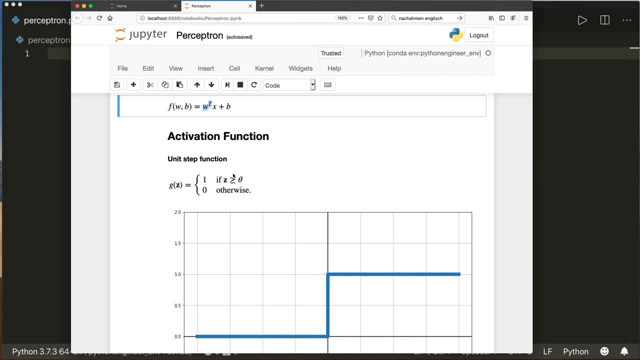 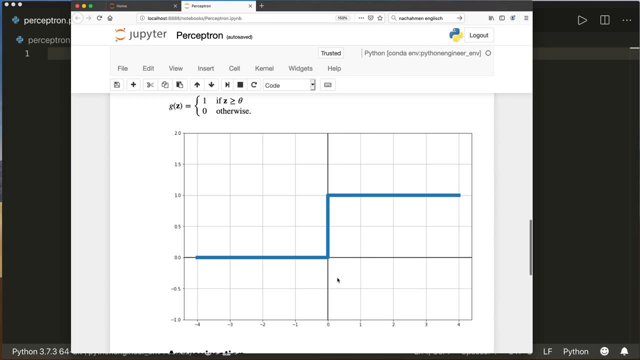 input reaches a certain, a certain threshold, or zero, otherwise. So in this picture, the threshold is zero. So if the input is larger than zero, then the output is one and otherwise it's zero. And now this is all we need to model the output. 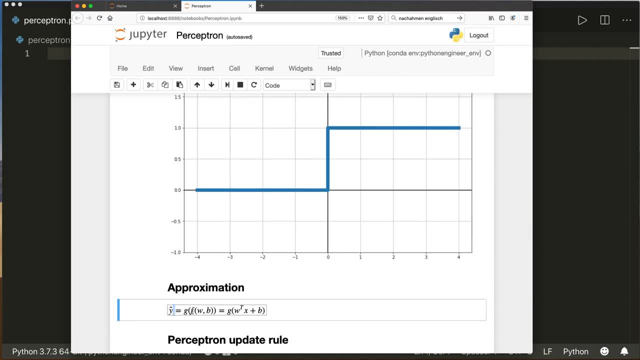 And now the whole output is looks like this. So first we apply the linear function, and then then we apply the activation function, And now we have to come up with the weights and the bias, And for this we use a simple update rule that is called the perceptron rule. So 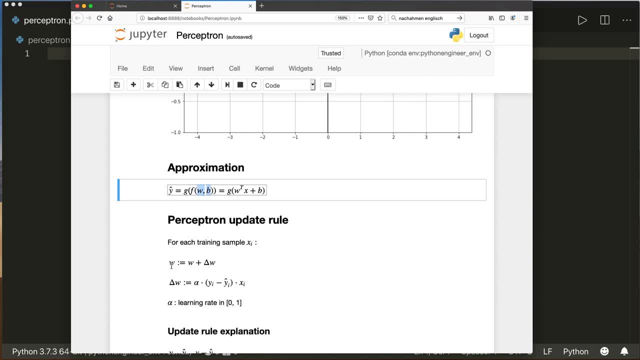 we look at each training sample x, i And for each training sample we then apply the update step And this is defined as the new weight is the old weight plus the delta weight, And the delta weight or delta w is defined as alpha times: the actual label minus the predicted. 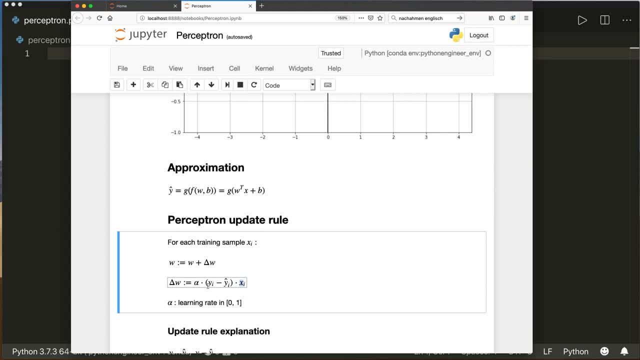 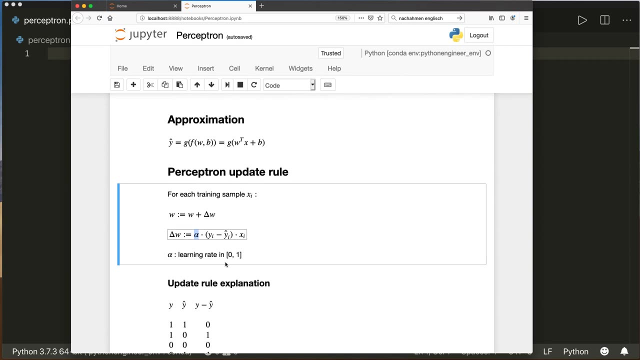 label times. the training sample x, And here alpha, is a learning rate between zero and one. So this is just a scaling factor. And now let's have a look at what this update rule means. So let's have a look at the four possible cases in a two class problem So our output can be one, the actual label can. 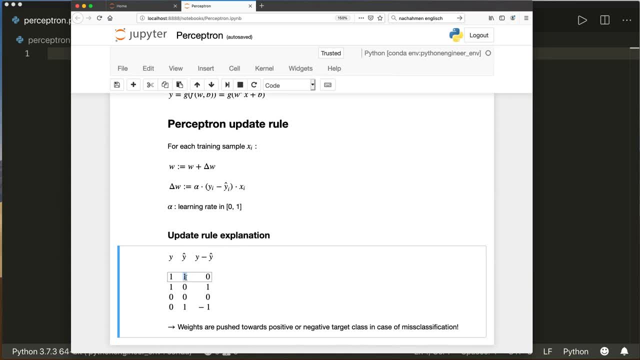 be one and the predicted label is also one, then the difference is zero, So we have no change for our weights here. And the same is if the actual class is zero and the predicted class is also zero, So correctly classified, then the difference is zero And again no change for our weights. But now what happens? 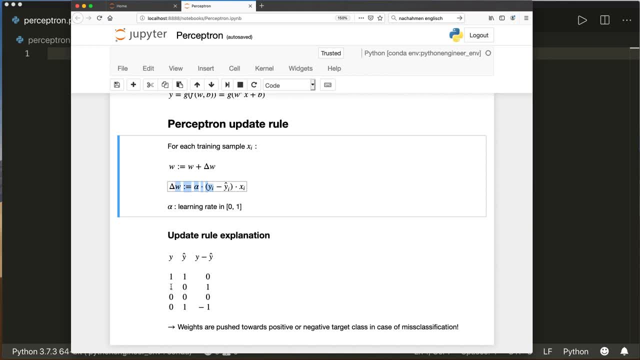 if we have a misclassification, So if the actual class is one and the predicted class is zero, this means that our weights are too low. And then we see that the difference is one, So our weights are increased here. And if the actual class is zero and the predicted 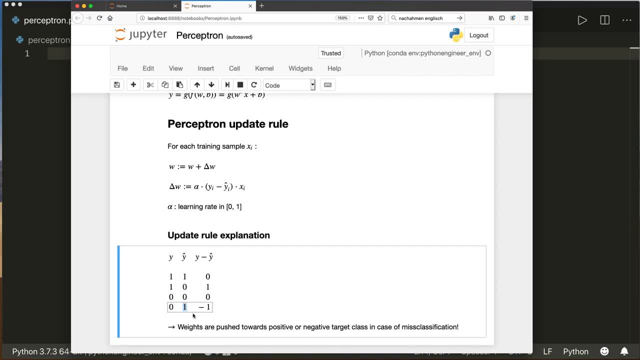 class is one, then our weights are too high And we see that the difference is minus one, So then our weights are decreased, So the weights are pushed towards the positive or negative class in case of a misclassification, And this is a simple and intuitive rule. but 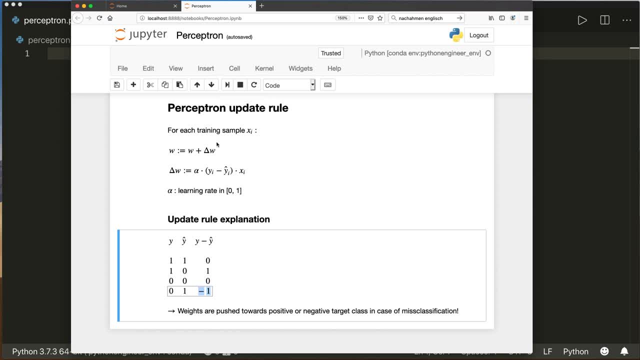 it works And this is all we need. So we look at each training sample and then apply the update rule, And then we do this a couple of times, So we iterate for a certain number of iterations And then we have the final weights and are done. So this is all we need to know And 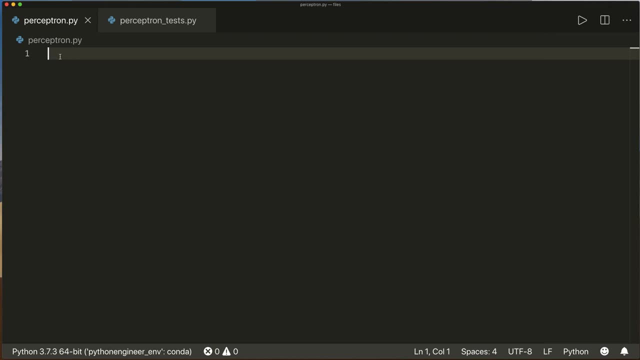 now we can get started and implement it. So first of all, of course we use numpy, So we import numpy s and P, And then we create a class and call it perceptron. perceptron And it gets an init method, of course, And here it has self and it gets the learning rate And I 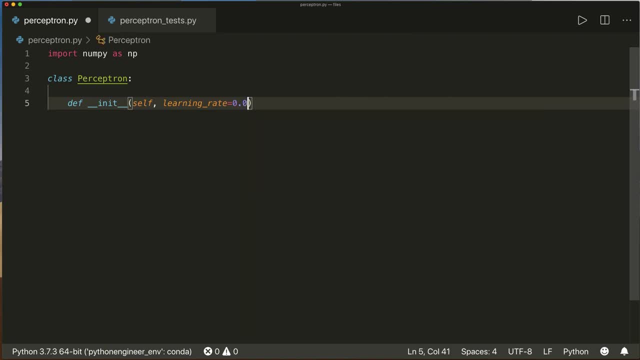 will give this a default of 0.01.. Then it gets a number of iterations, So an iter. and I will also give this a default, let's say 1000,. then I will simply store them. So I will say: self dot l? r equals learning rate and self dot n iter s equals an iter. 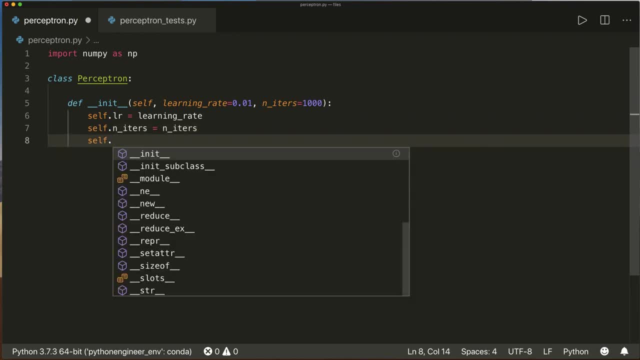 s. then we create a deactivation function. So let's say self dot, activation funk equals. And now let's create this here And, as I said, the activation function is simply the unit step function. So let's call this unit step funk with self and an input x. 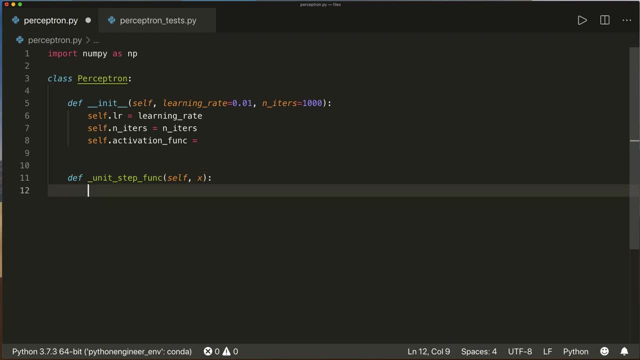 And we could simply say: return One if x is larger or equal than zero and else return zero. But we see later that we this would only work for one single sample. But we see later that we want to apply the activation function in the predict method for all the test samples. So we want to apply. 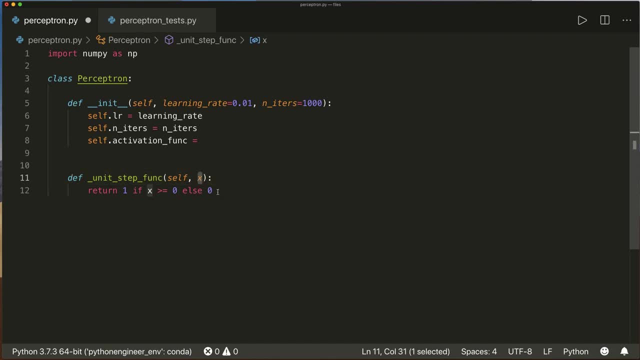 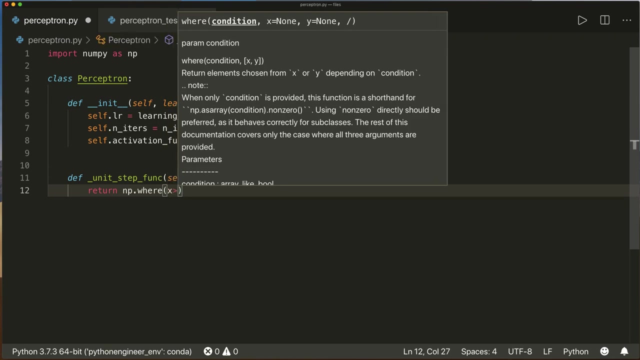 this for a Nd array as well, And for this we can use a simple function that is called numpy dot where. So we return numpy dot where, and this will get a condition- so x is larger or equal than zero, And if the condition is true, then we return one and otherwise zero. So this: 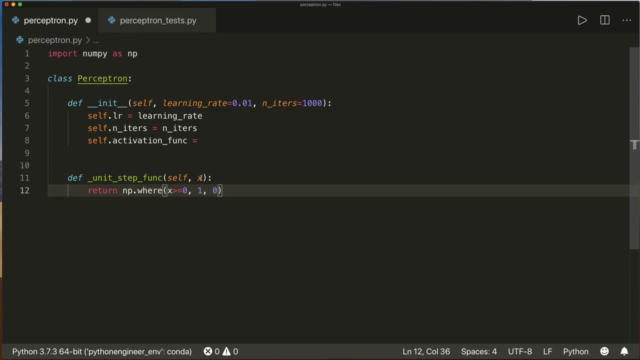 will work for one single sample, but also for a multiple samples in one vector. So now this is our activation function. So now we can say: self dot activation funk equals self dot unit step funk. And now let's also create the weights. say self dot weights equals none and self dot bias equals none. So now that 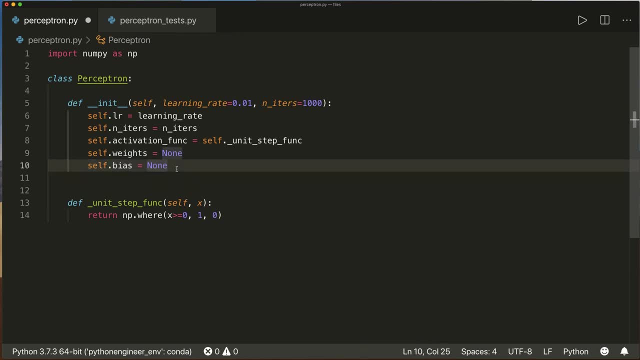 we know that we have to implement them or get them. And now we implement two functions. As always, we implement the fit and the predict method. So first define the fit method And then we define the predict method with x and y. So this gets the training samples and the 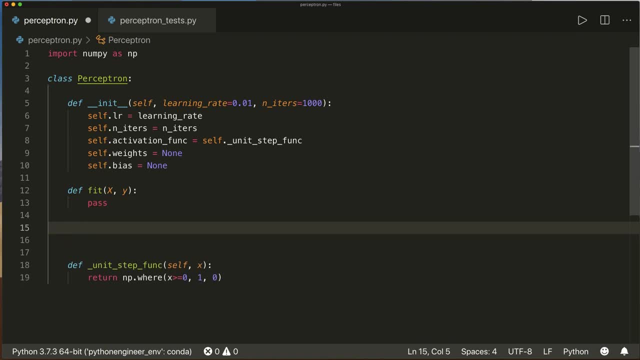 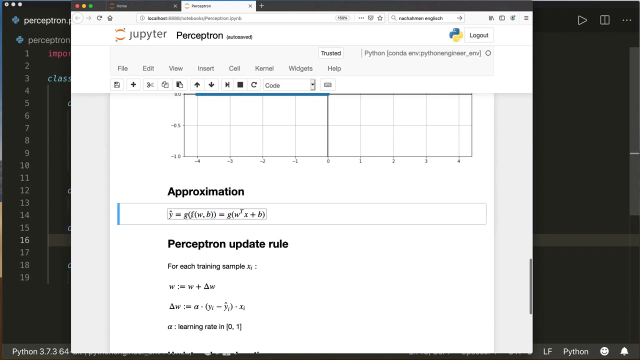 training labels And then, of course- oh, I forgot- the self. And then we also define the predict method, which gets self, and then the test samples. And now we start with this predict method, because this is self Very simple. Let's have a look at the approximation of our output again. So here, first we apply. 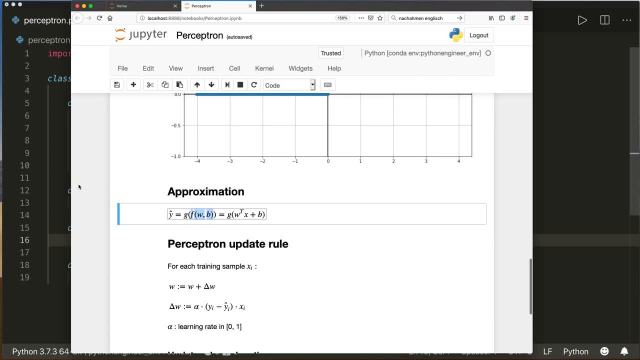 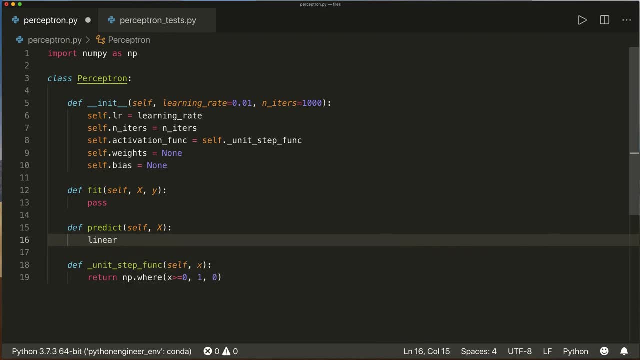 this linear function and then the activation function. So let's do this. So first the linear function. so let's say linear output equals, and this is: w transpose times x plus the bias, And w transpose times x plus the bias, And then we have the linear function, And then 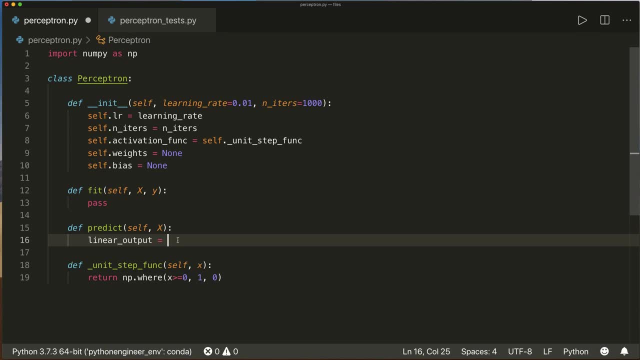 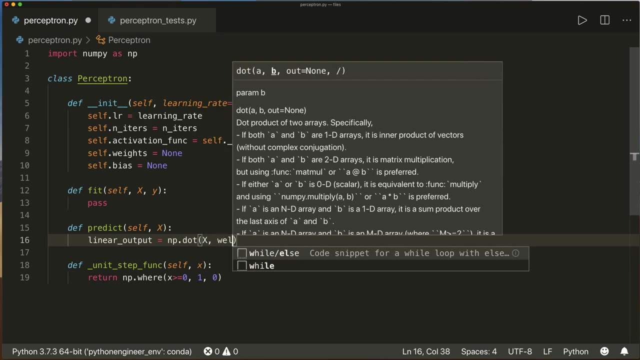 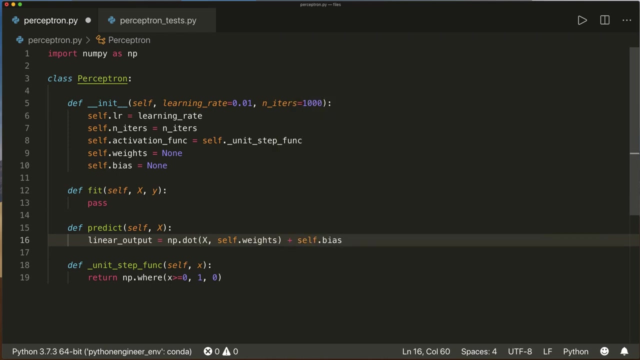 w transpose times. x is nothing else but the product. So we can use numpy dot of x and self dot, self dot weights plus self dot bias. So now we have the linear function And now we apply the activation function. So we say y predict, that equals self dot activation. 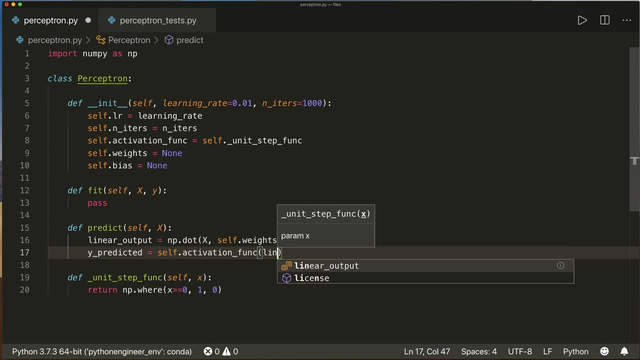 function And as an input it gets the linear output here, And then we simply return the y predicted. So this is the whole predict method. And now let's jump to the fit method. So first of all let's get the dimensions of the x vector. So this is an ND array of size m times n. 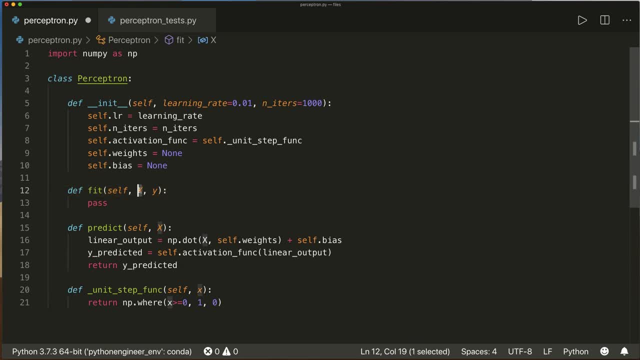 where m, or the number of rows, is the number of samples and n, or the number of columns, is the number of features. So we say n samples and n features equals x dot shape, And now we in it our weight. so we have to give them an initial value And we can simply 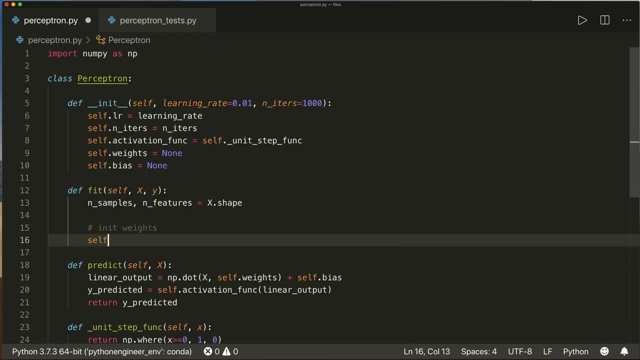 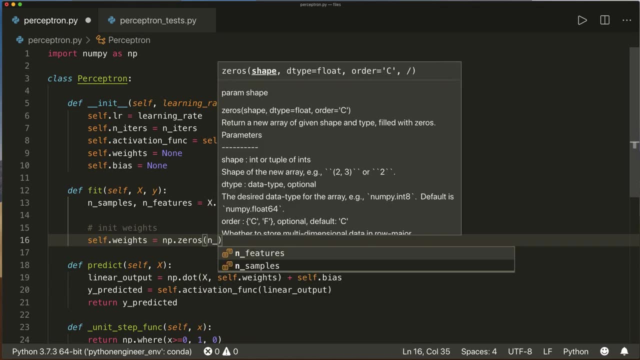 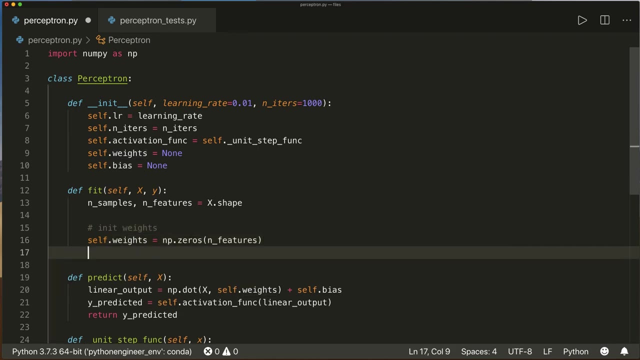 set them to zero in the beginning. So we say self dot weights equals numpy dot zeros of size, number of features. So for each feature we put a zero here for our weight And also our self bias. this is simply zero. And now we can start. or one more thing we have to. 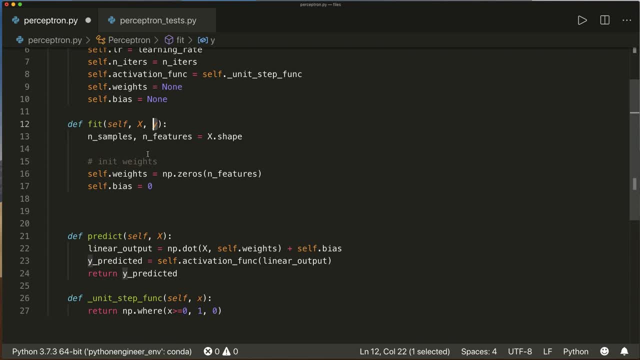 do is we want to make sure that our Y only consists of classes zero and one. So let's say y underscore equals, and now let's convert all the values to zero or one, if this is not already the case, So we use list. 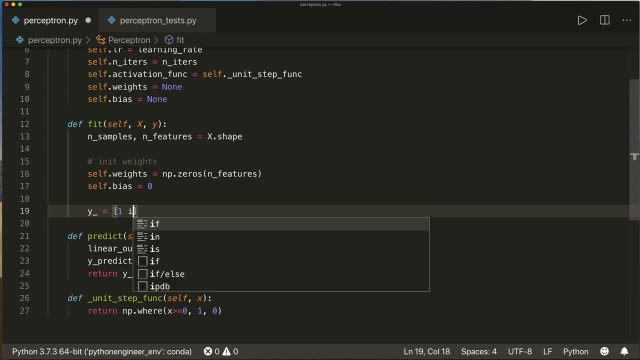 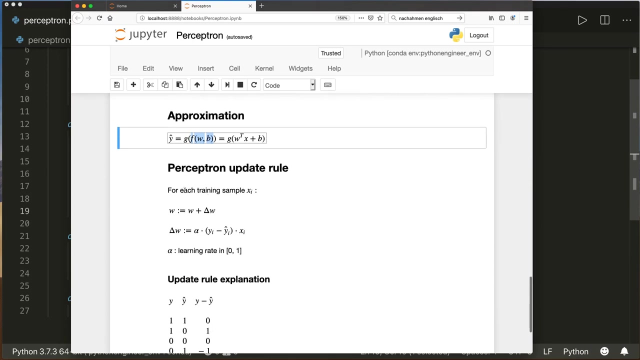 comprehension for this. So we say one: if I is larger than zero, else it's zero. four: I in y, And now let's convert this to numpy array. So now we have our y And now we can start to training. So let's again have a look at this update rule. So we want to look at 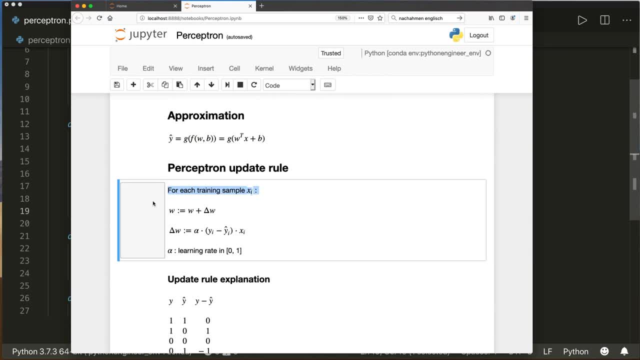 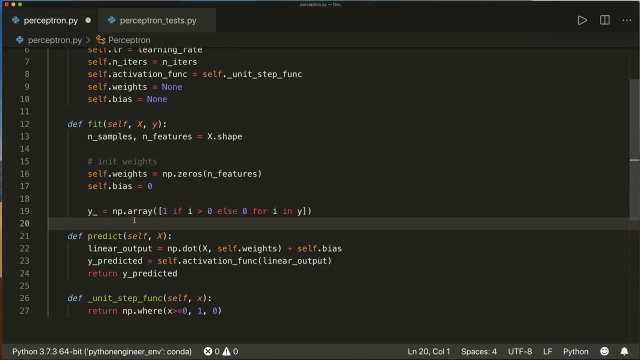 each training sample, And we also want to do this a couple of iterations. So we need two for loops here. So let's say the first one for underscore, because we don't need this in range self dot n itters. So this is the number of iterations we defined and then our 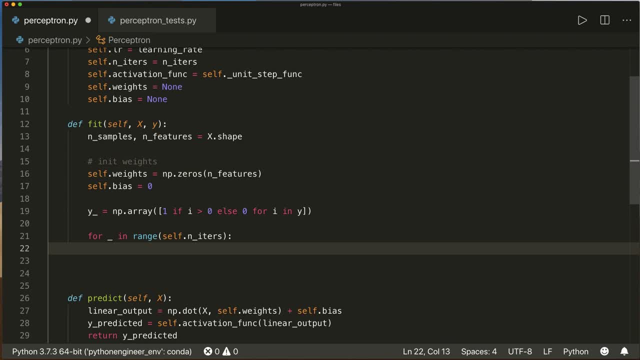 second loop, And for this I use the enumerate method so I can say for index and also x, y in enumerate x. So I want to iterate over the training, training samples, and the enumerate function will give me the index and then also the current sample. So these are our two loops. 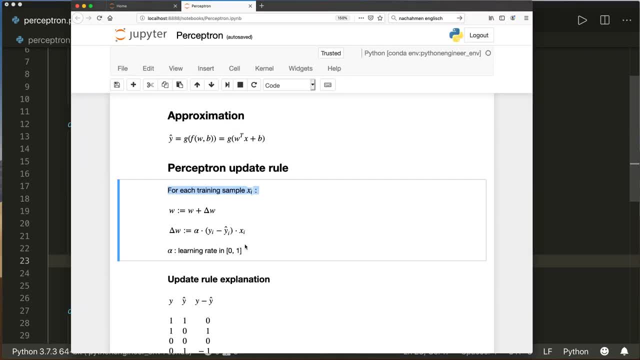 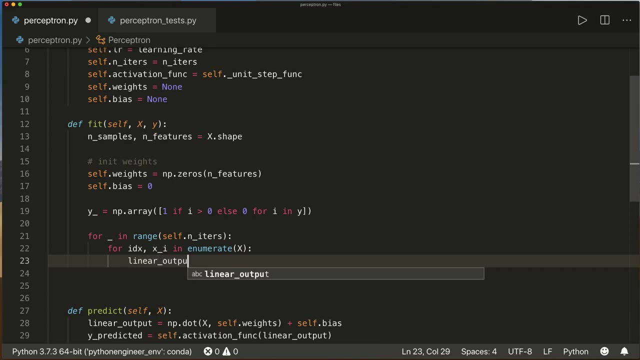 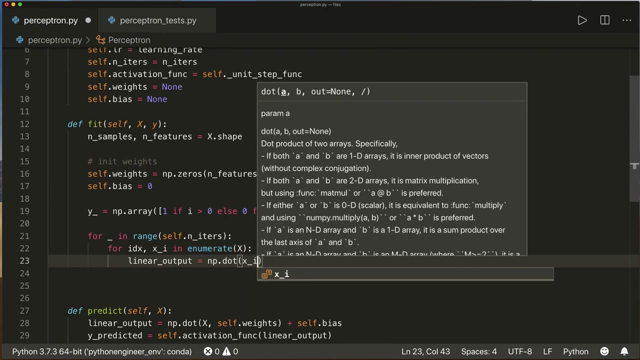 And now, sorry, let's apply this update rule. So let's again. we have to calculate the predicted value and then apply the update. So let's say, the linear output equals numpy dot of the current sample and our self dot weights plus the self dot weight. So let's say we 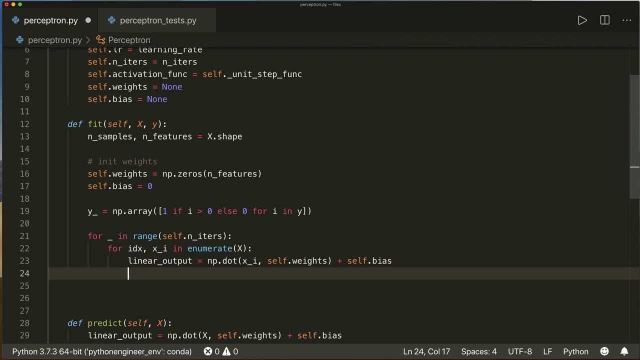 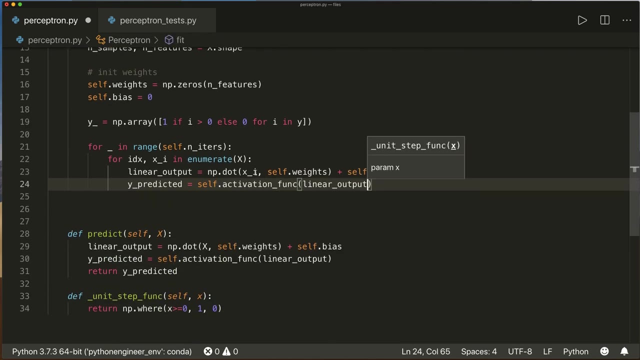 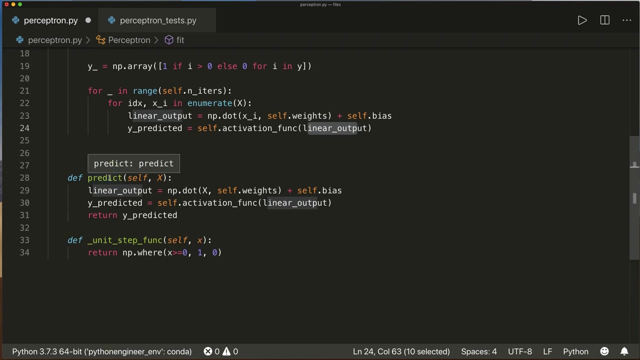 have the self dot bias, then we apply the activation function and get the predicted value. So y predicted equals self dot, activation function of the linear output. So here we can see that in this case we use it for only one sample And here down in the predict method: 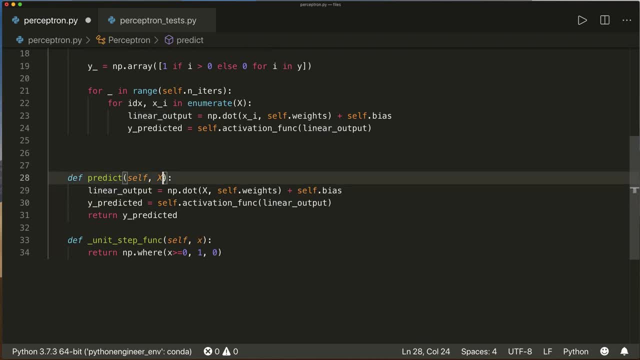 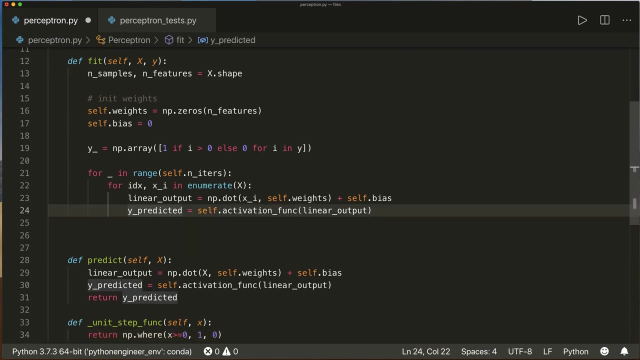 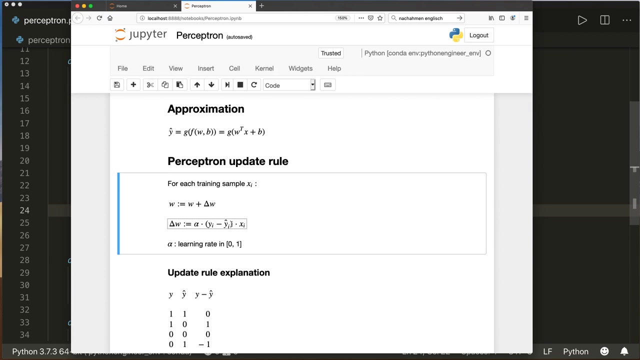 we use the activation function for multiple samples And that's why we need this numpy where function here in our activation function. So yeah, and now let's continue. So now we have our predicted y And now let's have a look at the formula again. So we have the learning rate, times the difference and then times. 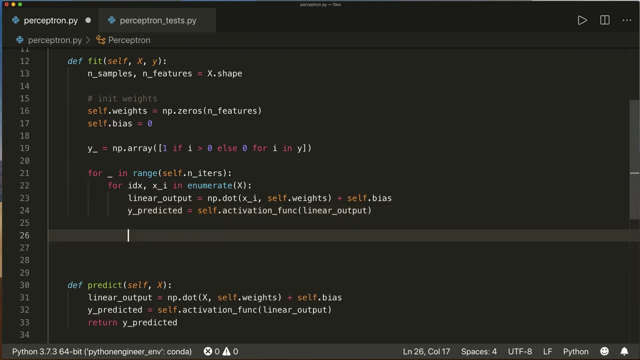 x. So let's call this: update equals self dot learning rate times, and here we have the actual label, So y underscore of this current index minus y predicted, And then we say self dot weights plus equals update times: x, i and self dot bias. 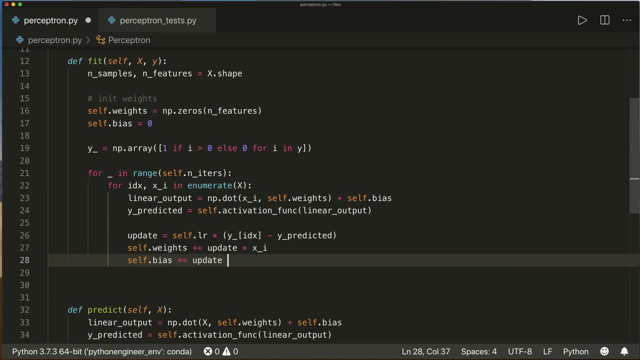 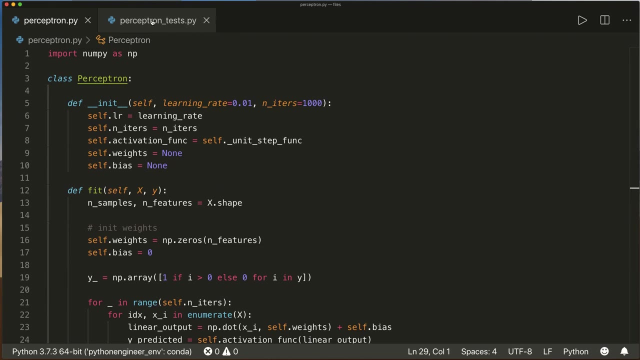 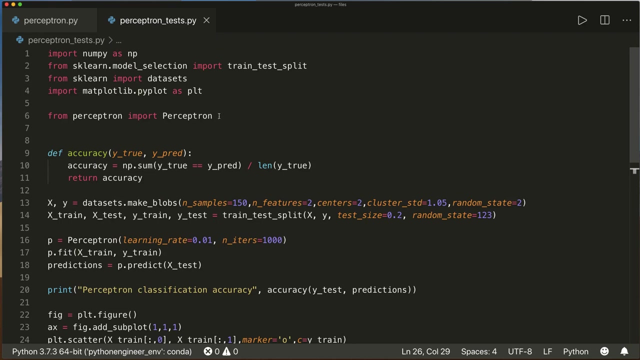 So we don't need this times one, And now we are done. So this is the whole implementation of the perceptron, And now let's test this. So here I've written, I've already written- a little test script here. So I import the perceptron here And then I will create two.